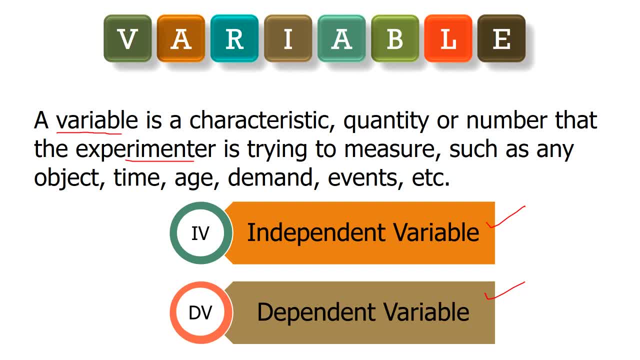 variable is a variable which is being measured Further. an independent variable determines the dependent variable, and so the dependent variable relies on independent variable for its value. For example, the value of a car is dependent on the age of the car. So here the dependent variable is the value of the car, while the independent variable is the 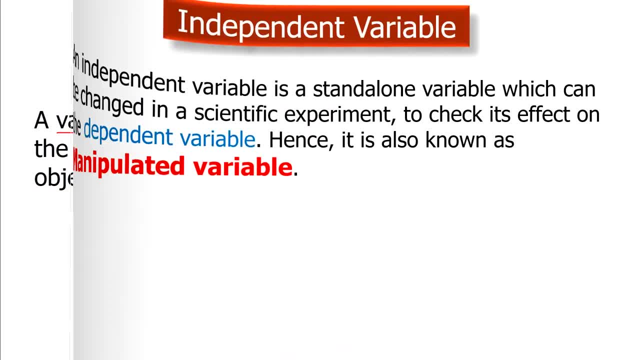 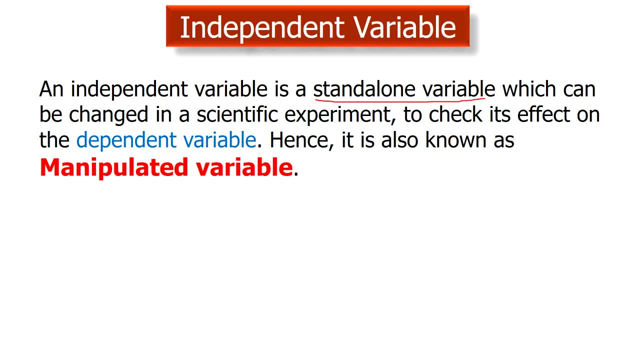 value of the age of the car. Independent variables. An independent variable is a stand alone variable, meaning that it is a variable whose change is not affected by any other variable in an experiment. The independent variable is either changed or controlled in a scientific experiment by 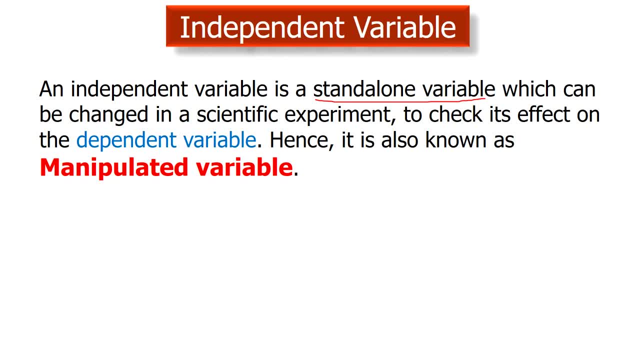 the experimenter or it changes on its own due to circumstances. The experimenter checks its effect on the dependent variable. an independent variable reflects the cause or reason for an outcome. further, as it indicates the quantity which is being manipulated in an experiment, it is 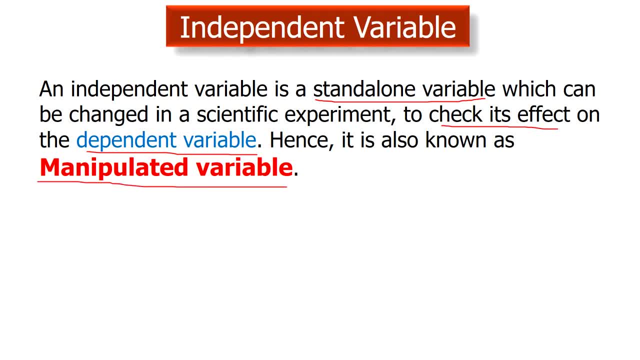 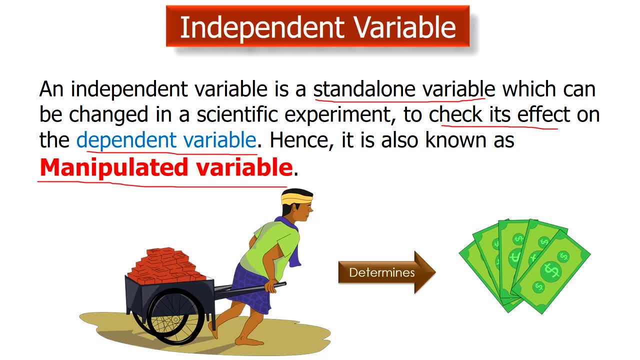 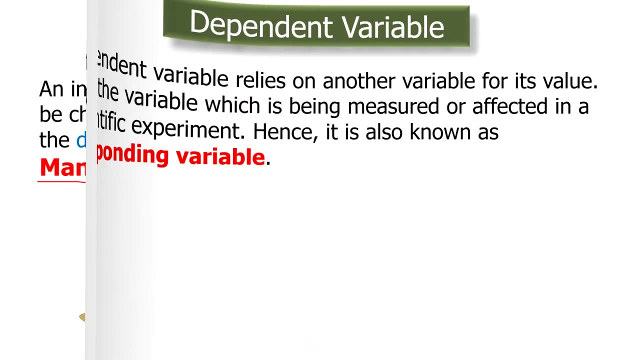 also called as manipulated variable. now let's take an example. the amount of wages earned by a labor depends on the hours he has worked. hence the working hours will determine his pay for the day. so it is the independent variable dependent variable. dependent variable is the variable which relies on another. 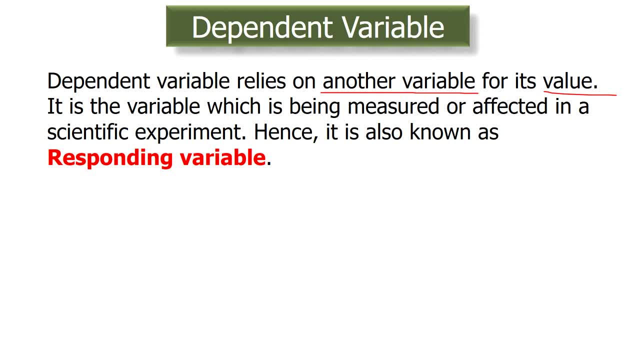 variable for its value. it is the variable which is being measured or tested in an experiment. it indicates how the change in independent variable has affected the dependent variable. that is why it is also known as responding variable. in a scientific experiment, the experimenter changes the value of. 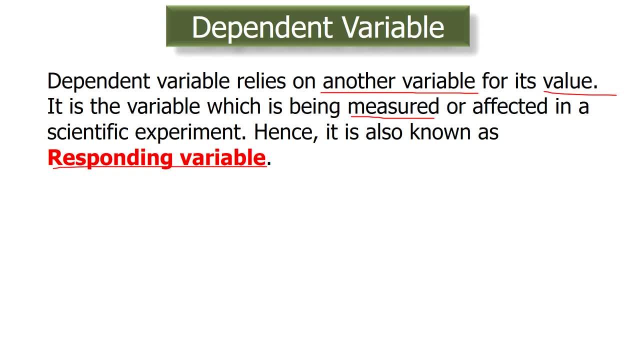 independent variable so as to observe and record its effects on dependent variable. hence one cannot get the value of dependent variable without independent variable. so the independent variable denotes the if part of hypothesis, whereas dependent variable is the then part of the hypothesis. now let's take an example. the calories burned by a person depends on the hours. 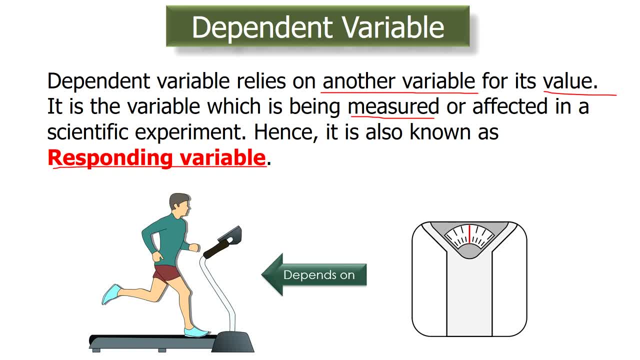 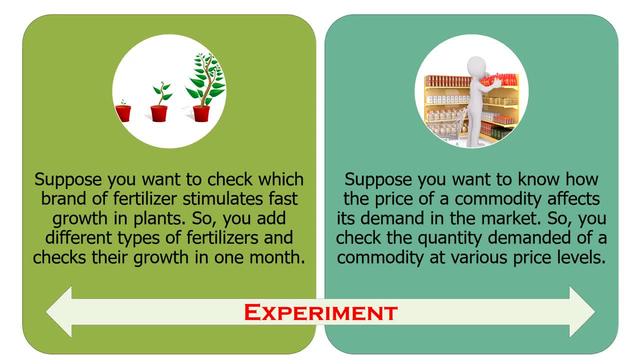 spent on exercising. so here the calories burned would be. the dependent variable means the plant height which is being observed and recorded. experiment two: suppose you want to know how the the price of a commodity affects its demand in the market. So you check the quantity demanded of a commodity at different price levels. In this case the independent variable is the. 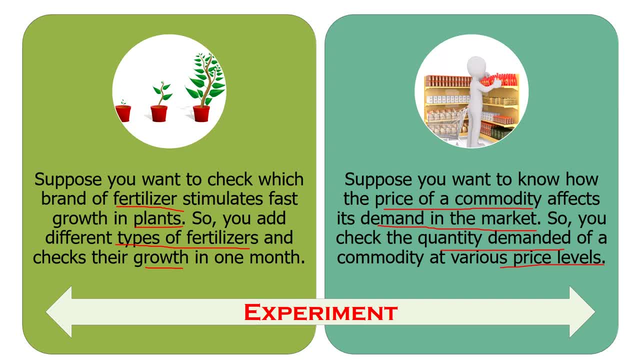 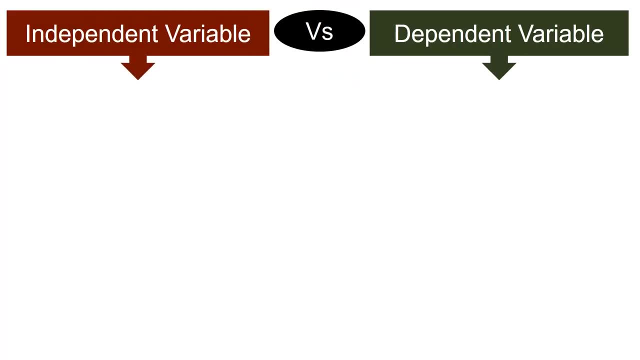 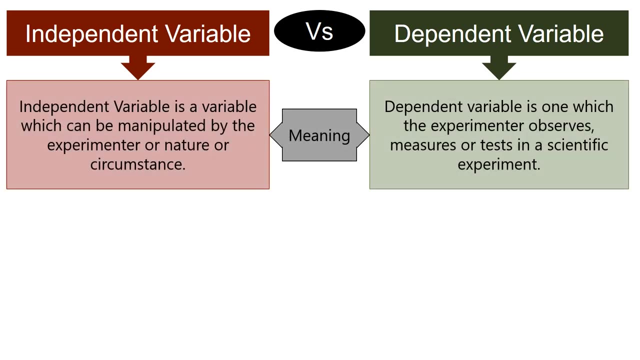 price, which is being manipulated during the experiment, whereas the dependent variable is the demand for the commodity which is affected by its price. Now come let's discuss the differences between independent and dependent variable Meaning: An independent variable is a variable which can be manipulated by the experimenter, or 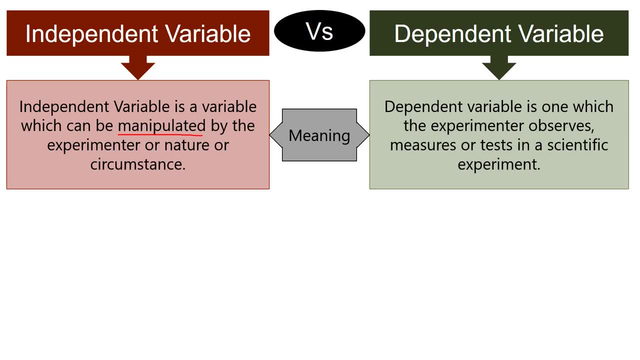 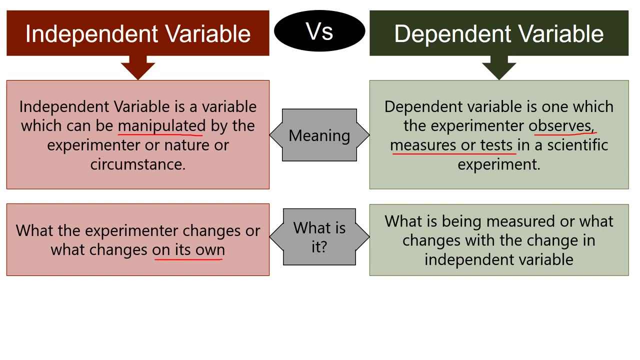 nature or circumstance during the experiment. As opposed, dependent variable is one which the experimenter observes, measures or tests in a scientific experiment. An independent variable is the variable which the experimenter changes or what changes on its own. Conversely, a dependent variable is the variable which is being measured or what. 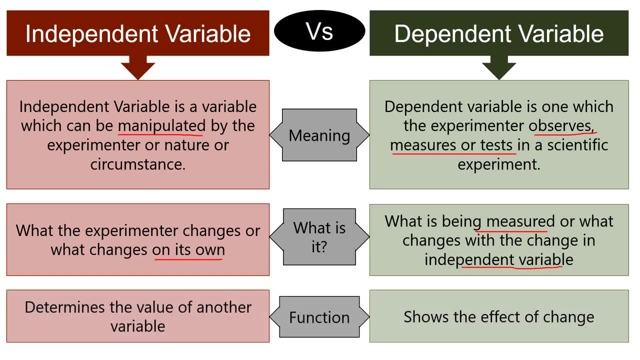 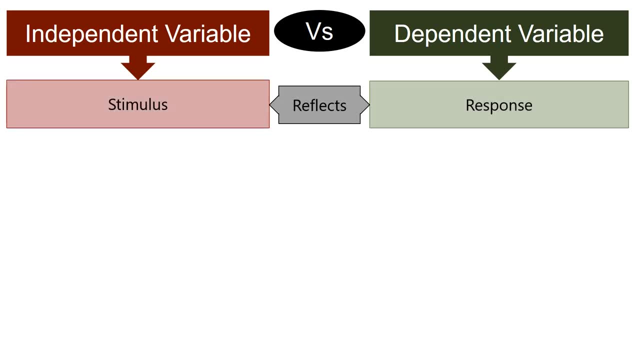 changes with the change in value. While the independent variable determines the value of another variable, dependent variable shows the effect of change of independent variable on the dependent variable. Next, an independent variable is the stimulus which causes the change in another variable. Conversely, dependent variable reflects the response, which shows the outcome or effect. 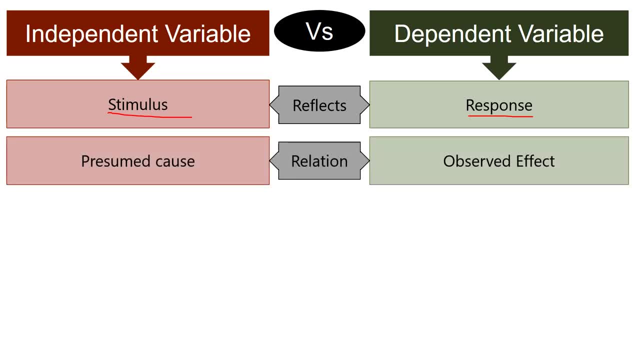 of something. When it comes to relationship, independent variable is the presumed cause. on the other hand, dependent variable is the observed effect. further, the independent variable is also called as experiment controller, because it is the variable which controls the entire experiment. on the contrary, the dependent variable is also known as experiment.